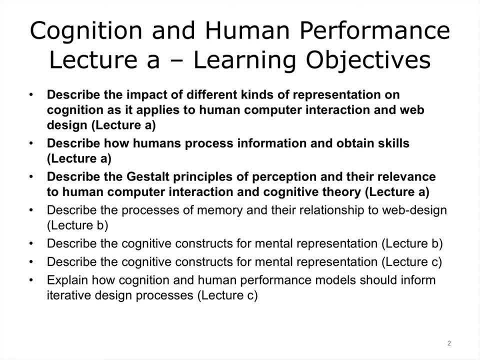 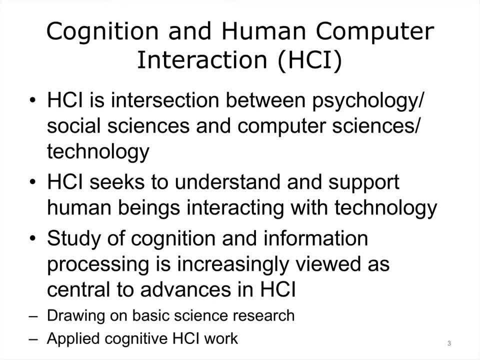 Describe the Gestalt principles of perception and their relevance to human-computer interaction, and how human-computer interaction can be applied to human-computer interaction and cognitive theory. Given that this is a course on usability and human factors, why should we be concerned with human cognition or theories that largely arise out of the psychological literature? 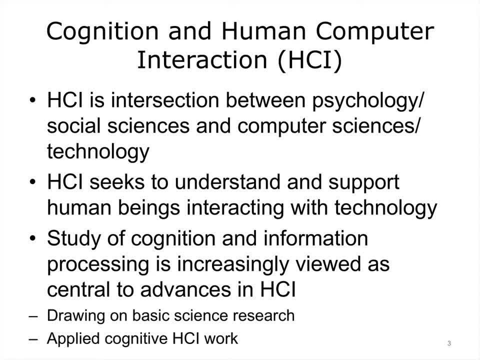 There are two answers to that question. The first is that the computing experience is a deeply human endeavor that engages the cognitive and perceptual systems. The second is that the disciplines of human HCI and human factors draw heavily on both basic and applied research. In this particular set of lectures, 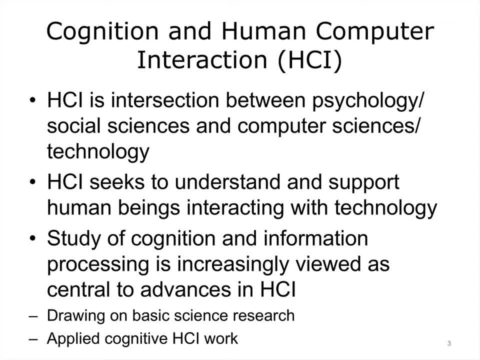 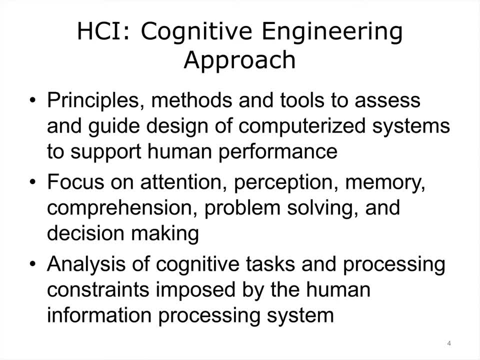 we will draw on cognitive theories in view to understand the way it affects the computing experience in health care contexts. The cognitive engineering approach is one of the most influential in HCI and human factors. Don Norman, who we discussed previously, is one of the pioneers of this approach. 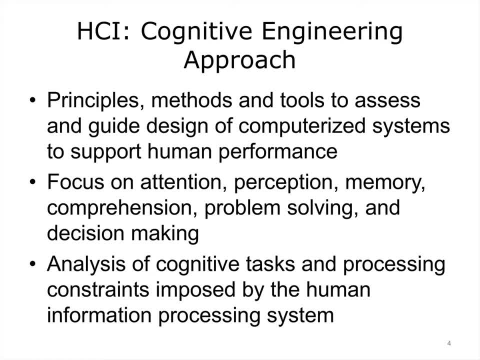 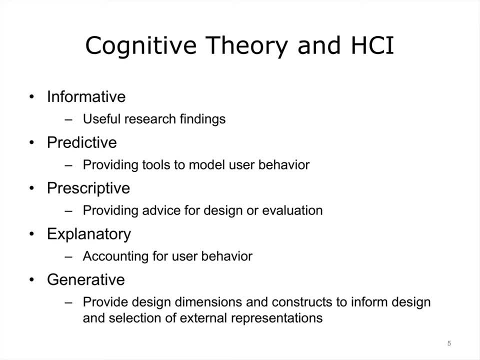 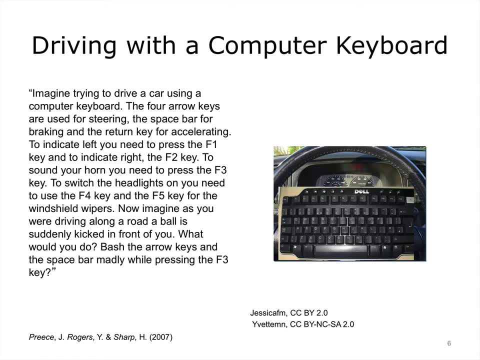 Cognitive engineering places a strong emphasis on cognitive, perceptual and cognitive learning. Cognitive engineering places a strong emphasis on cognitive, perceptual and cognitive learning. no attention to human capabilities. This example was drawn from a text by Jenny Preece and colleagues. Imagine driving with a keyboard instead of a steering wheel. That seems like. 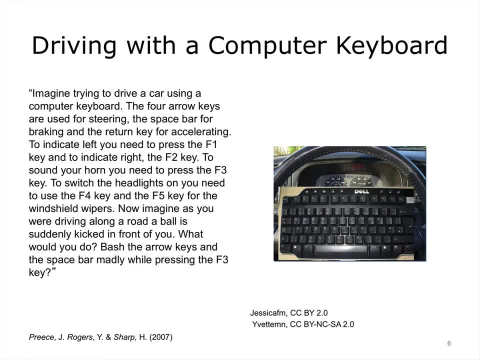 an absurd idea, but it serves to highlight how some tools can be so poorly situated for a particular purpose, given human information processing capabilities and their limitations. Keep in mind that this is just an example. Please don't try to drive using your keyboard on the. 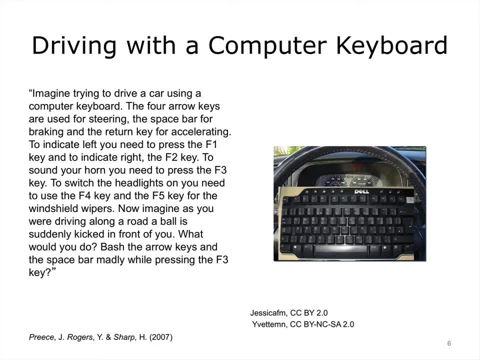 highway. Imagine trying to drive a car using a computer keyboard. The four arrow keys are used for steering, the space bar for braking and the return key for accelerating. To indicate left, you need to press the F1 key and to indicate right, the F2 key. To sound your horn, you need. 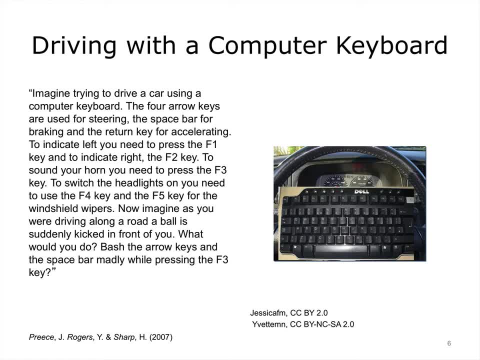 to press the F3 key To switch the headlights on. you need to use the F4 key and the F5 key for the windshield wipers. Now imagine, as you are driving along a road, a ball is suddenly kicked in front of you. What would you do? Bash the arrow keys and the space bar madly while pressing the F3. 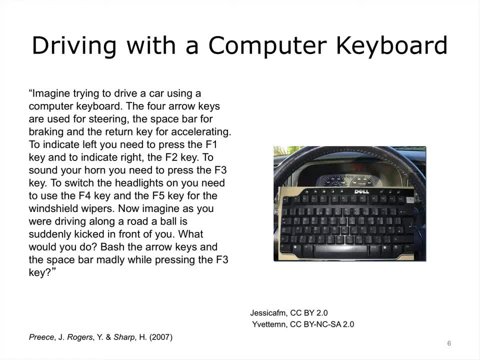 key. This example serves to illustrate that perceptual, motorist and cognitive responses can't possibly be effectively supported by such tools. This is a case where safety would be clearly compromised. Although the example is a bit extreme, there are many instances in which 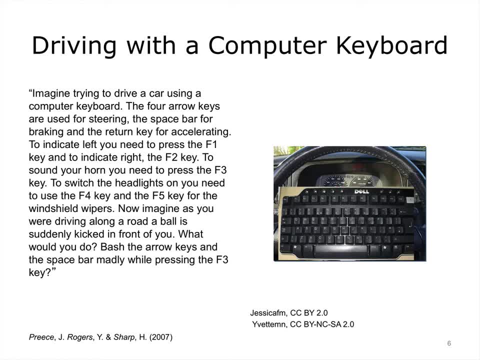 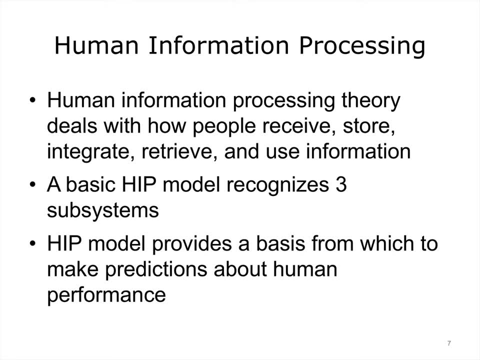 tools completely fail to exploit human capabilities and make tasks unnecessarily difficult. Human information processing theory deals with how people receive, store, integrate, retrieve and use information. The basic model recognizes three subsystems: Perceptual system that processes incoming sensory information. Motor system controls action and physical behavior. 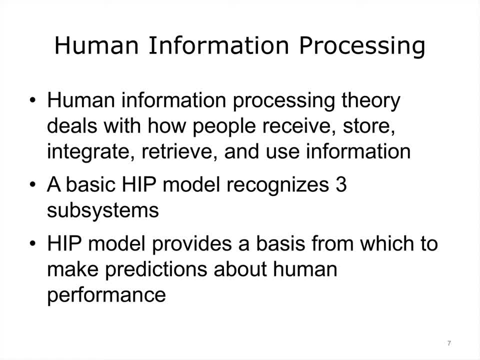 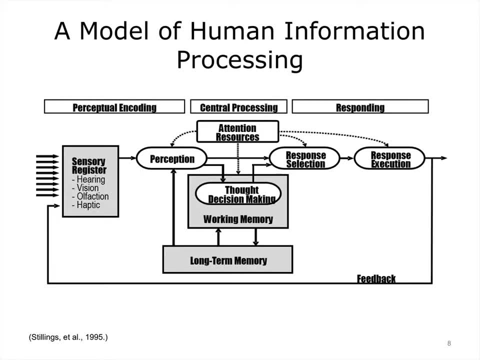 Cognitive system provides the processing that connects the two systems. We're going to briefly deal with different dimensions of the system. We're going to deal with different dimensions of the These subsystems. This is a simplified model of human information processing. We can characterize it as a 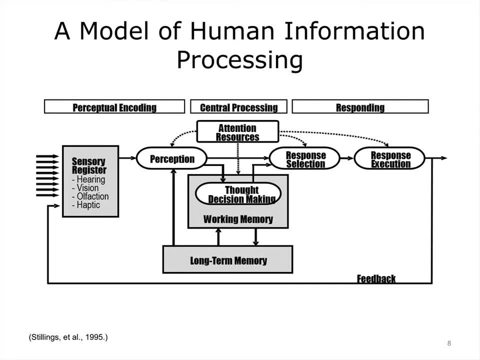 multi-stage process that begins when our senses, such as vision and hearing, come into contact with stimuli in the world. A very small percentage of these stimuli are passed along for further processing. Our attention mechanisms determine what information requires a particular kind of response. For example, if you're driving a road, you're going to need to pay attention to the. 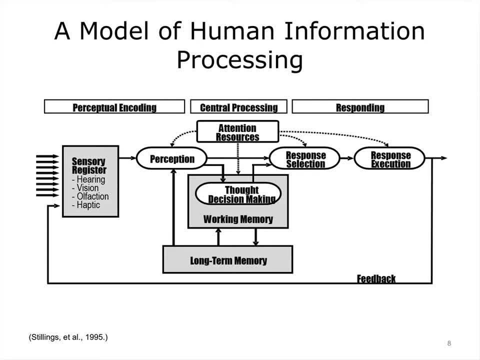 driving and you suddenly see a ball in the middle of the road, you will immediately swerve without giving it any thought. It's a simple reflex action. However, if you come across an email that offers you a career opportunity, it will require some deliberation and decision making Information. 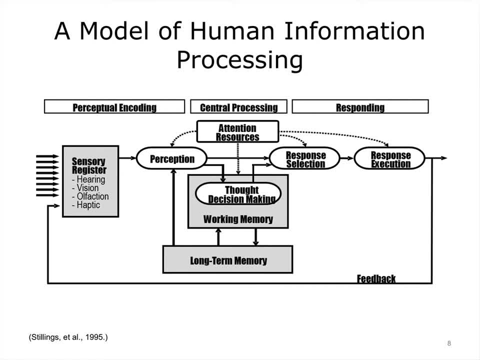 from the senses is transferred to the different memory systems for either immediate processing or long-term action. It's important to keep in mind that this diagram is an idealization and a simplification of a very complex system, But this will suffice for the purposes of discussion. To reiterate, it's useful to distinguish three. 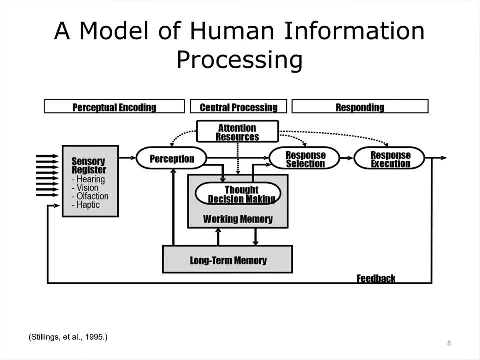 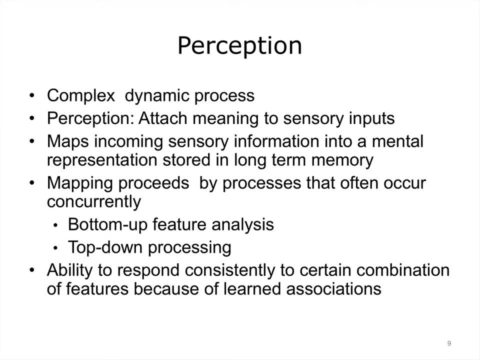 subsystems, including perceptual mechanisms, central processing that gives meaning to perceptual input and a subsystem that supports action. Perception is a set of dynamic processes that attach meaning to sensory inputs. It maps incoming sensory information into a mental representation stored in long-term memory. A simple example is: 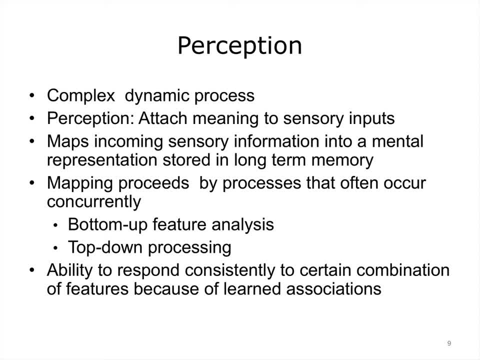 that when you are in a public space, you will react to a face you know, whereas you may not even perceive other faces that don't attract your attention. Bottom-up processing refers to the analysis of features that one would try to integrate into a whole. Top-down processing includes using knowledge. 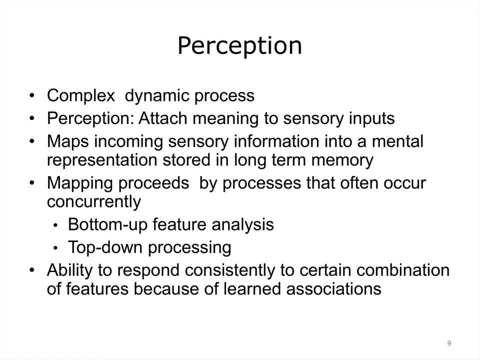 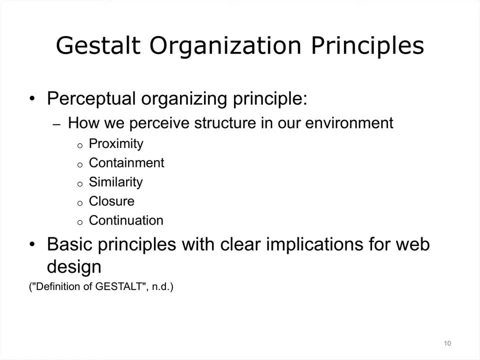 stored in long-term memory to recognize objects, people and events. A nice illustration of the implications for design, and web design in particular, are seen in gestalt: perceptual organizing principles Gestalt according to the Merriam-Webster. 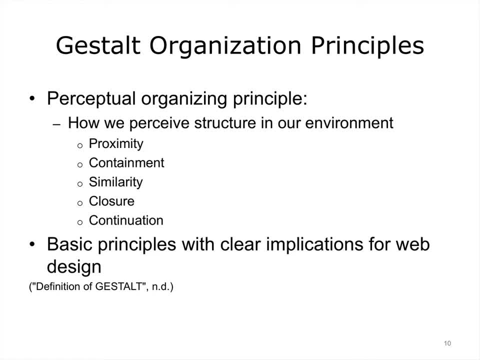 dictionary means: quote something that is made up of many parts and is yet somehow more than or different from the combination of its parts. Broadly, the general quality or character of something. end quote: Gestalt: perceptual organizing principles predict the way the 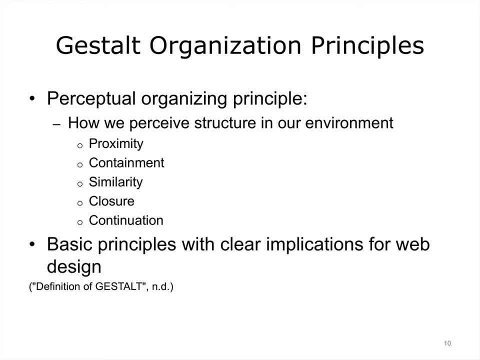 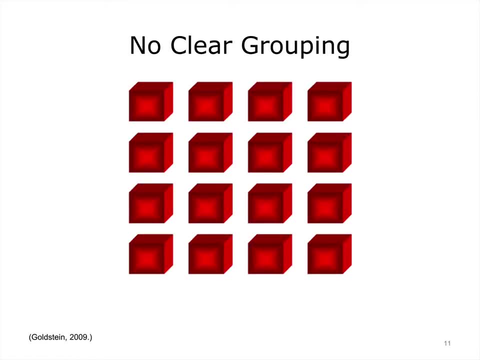 human perceptual system will react to objects we see in a display. Let's go through a series of examples. This illustration shows 16 blocks with no guidance on how to perceptually organize them. It makes it rather hard for viewers to follow. The proximity principles suggest that we perceptually group. 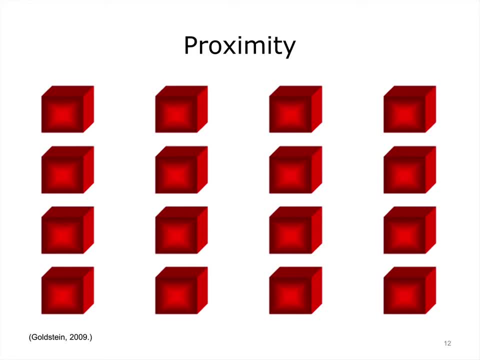 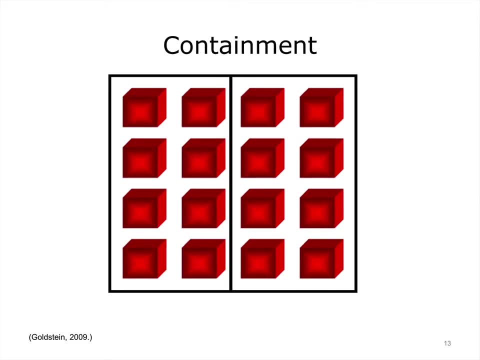 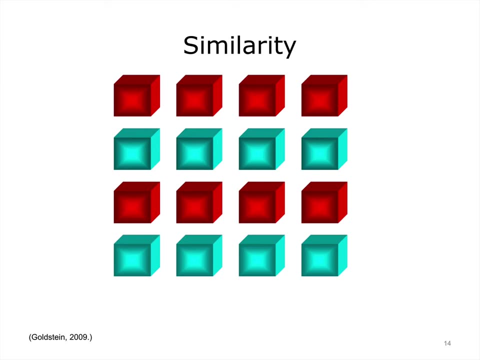 objects by their closeness to one another. We can clearly see four groups in this picture. If you put things inside of boxes or frames or inside borders, that suggests a way to group them. Color can be used to effectively partition a space and lets us know that they designate a type or 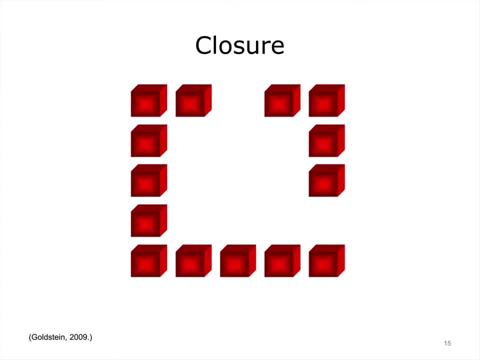 category. Humans have a natural tendency to see closure if a grouping suggests it. For example, the letters B and R are often handwritten in such a way that the semicircles in each letter do not appear to be fully closed, But people will typically not have any problem recognizing the letters for 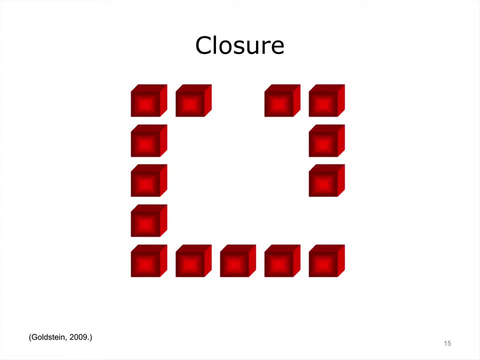 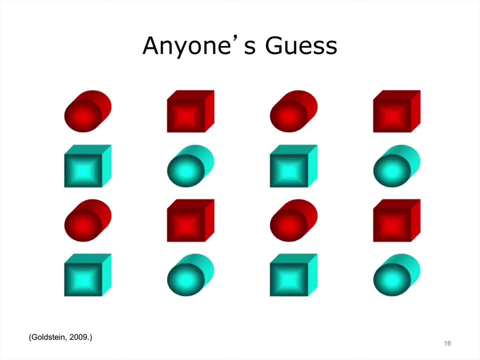 what they are. Of course, bad handwriting perceptually degrades them and makes that task all that much harder. Arbitrary arrangements of objects provide no clues to categorical grouping. A lack of categorical grouping makes it more difficult for us to make sense of a web page and or learn to use a system. 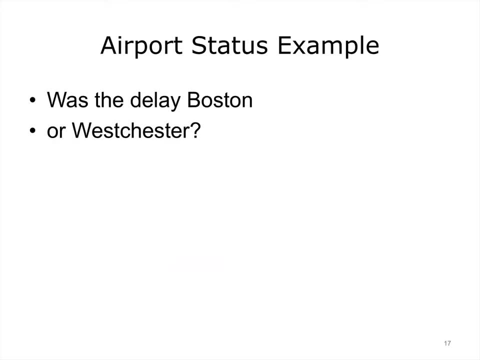 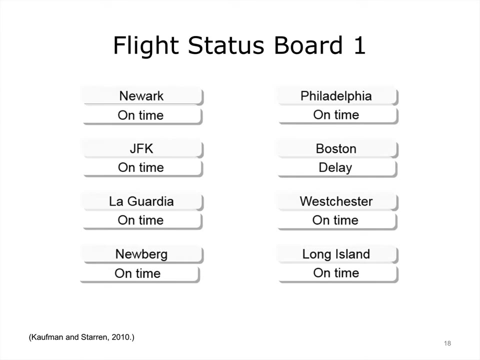 productively. Public displays are an important source of information. Let's imagine that you're waiting to go to Boston and you want to know if your flight is delayed. You would check out a flight status board. Schedule 1 offers you a neatly laid out screen, but it all looks the same. You need to serially scan. 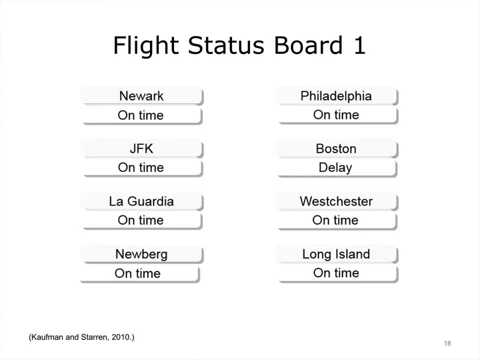 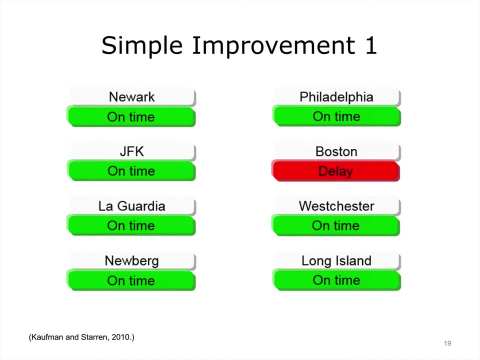 the board, that is, examine each entry one at a time to find the information you need. The color red offers a simple improvement, because one eye is immediately drawn to the delay. This slide simplifies the display and you can see that the display is now in the middle of the screen. 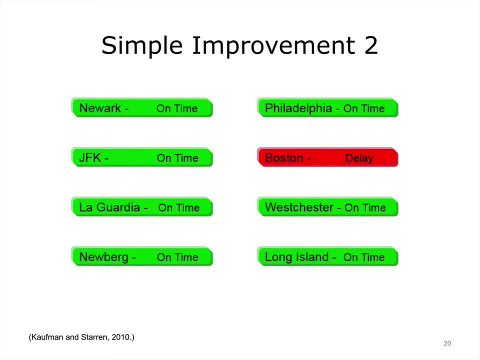 You can see that the display is now in the middle of the screen. You can see that the display is now in the middle of the screen. This slide simplifies the display and you can perceptually pick up the information even more effortlessly because you're presented with an integrated hole. 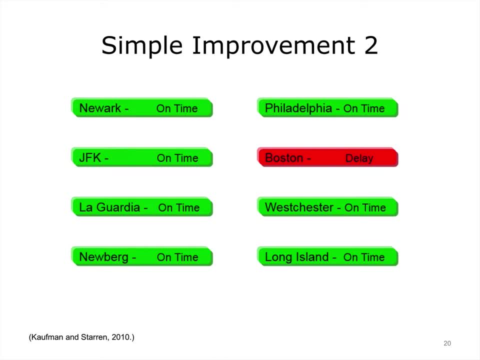 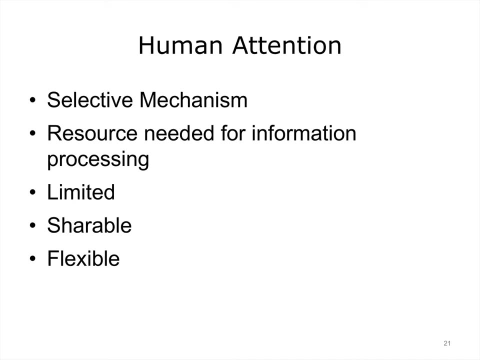 The perceptual and cognitive systems have less work to do. Attention mechanisms are used to allocate resources to the kind of work the cognitive system has to do. Attention resources are limited. You can share them across tasks if necessary. They are flexible. For example, multitasking requires divided attention. 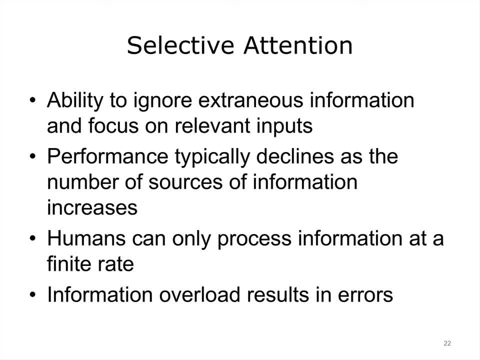 If you paid attention, or equal attention, to everything that your senses perceive, you would simply be overwhelmed. In fact, that can happen in stressful work environments. Humans can only process so much information over a period of time, and overload can result in errors. 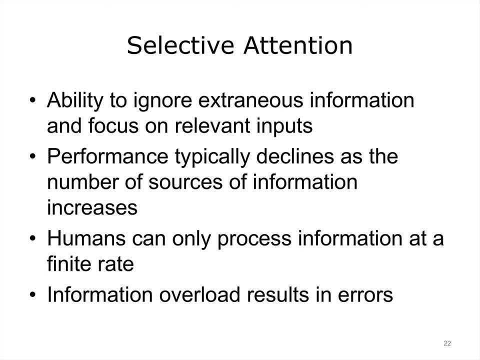 The four points on the slides describe both the potential of humans to employ attentional mechanisms productively and the downside of being confronted with a situation in which demands exceed capacity. Attention is a topic of importance in human factors work. Information overload is not an uncommon problem in a busy workplace and clearly evidenced in overcrowded hospital settings. 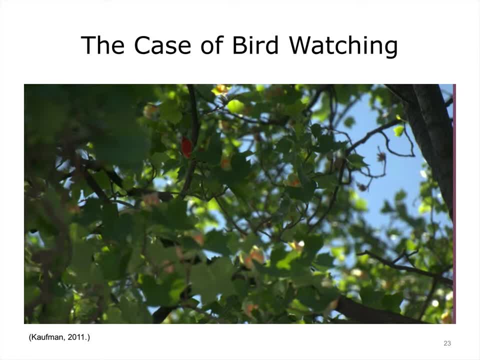 If you've ever had a birdwatching experience and you go out with a friend who is an experienced birdwatcher, he or she will spot things that you will not be able to see right away. You may have to serially scan through thick leaves before you see anything that resembles a bird. 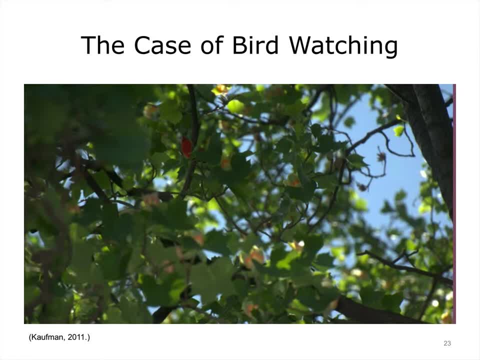 On the other hand, your bird-savvy friend can immediately attend to cues that are important, eg very slight movements, changes in light and will perceive signal to your noise. This is the computerized provider order entry screen that we have seen in previous lectures. 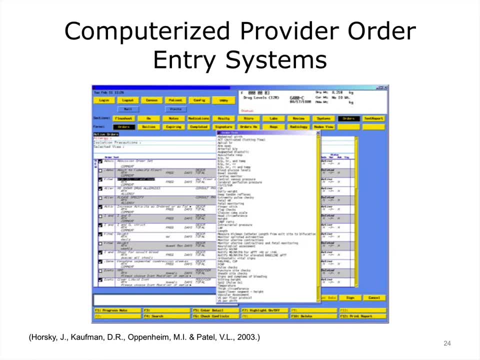 Notice that there is a very lengthy pick list of tests. If you have considerable familiarity with the Glasgow Como scale, then you may be able to more readily perceive it on this alphabetized list. If you're not, you will have much more work to do to find what you're looking for. 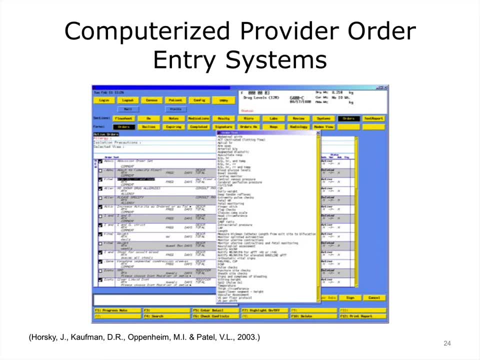 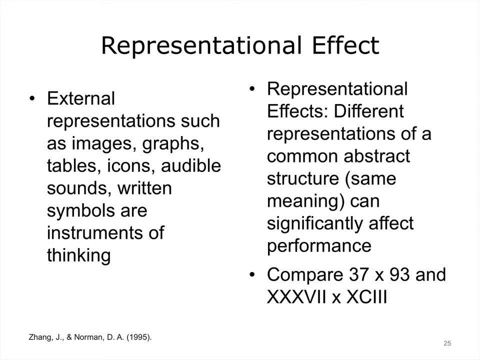 This picture exemplifies a very complex screen that supports an enormous range of functions. The display is cluttered and it can be challenging to make selections given the density of information. There is a widely documented and important phenomenon known as the Representation Effect. You can use different symbols to express the same idea. 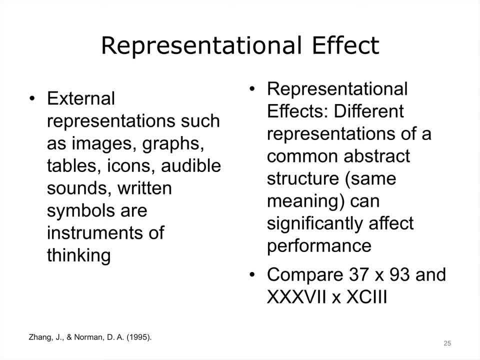 For example, if you want to communicate population growth in the state of Florida over the past 50 years, you can do so in words, in a tabular format or graphically, in many different ways. How it will be perceived depends in part on your purpose and on your audience. 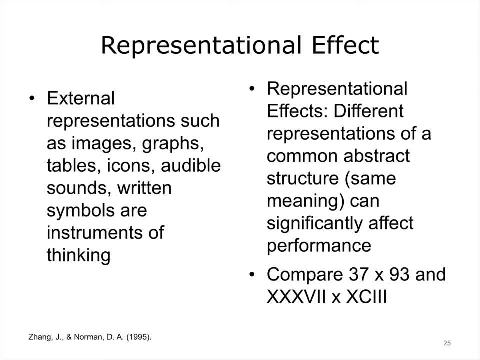 but these different representations of the same ideas or the same information will have significant perceptual and cognitive effects. Compare multiplying 37 by 93, and then consider using Roman numerals, XXXVII times XCIII, Even if you're very well versed in Roman numerals. 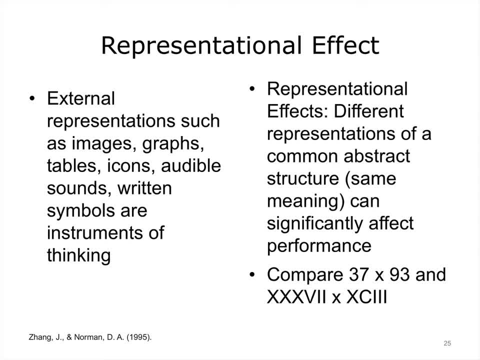 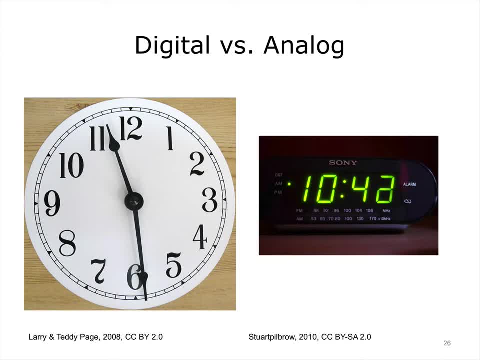 chances are, you will still find it difficult to multiply these numbers that way. We are all acquainted with both digital and analog clocks. If you want to know the time in a hurry, then you can quickly perceive the numbers on a digital clock. On the other hand, if you want to find out how much time you've spent surfing the internet, 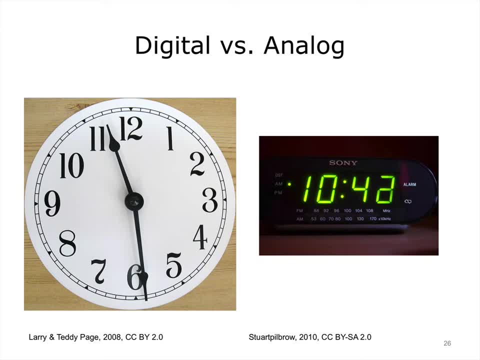 then you can quickly perceive the numbers on a digital clock. On the other hand, if you want to find out how much time you've spent surfing the internet, the analogue clock provides more resources for quickly perceiving that twelve minutes have elapsed since you started surfing. 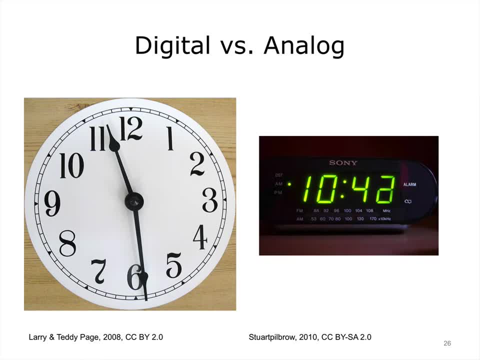 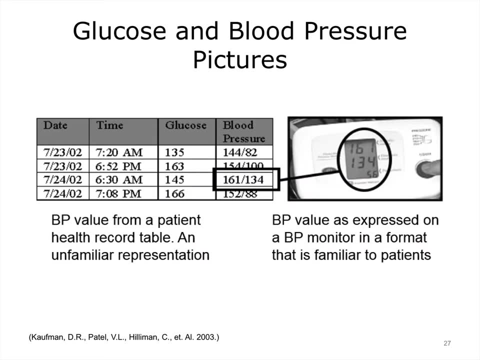 On a digital clock, such an inference involves a calculation. On a digital clock, such an inference involves a calculation, and even if it's a simple one will necessitate the use of more resources. Table Can support quick and easy look up and are a compact and efficient representational device. 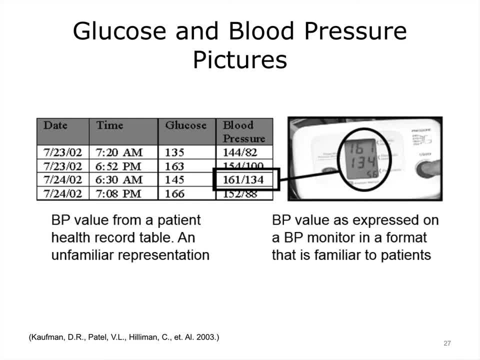 However, a particular external representation is likely to be effective. some population of users and not others. For example, reading a table requires a certain level of numeracy that is beyond the capabilities of certain patients with a very basic education. Numeracy refers to quantitative literacy. 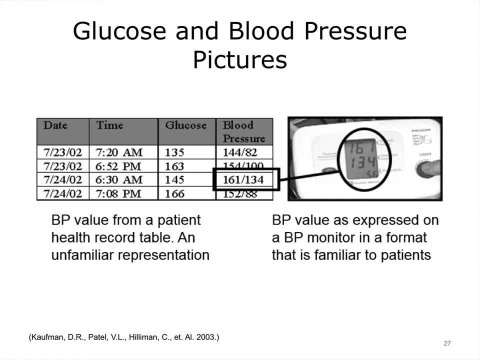 Research has shown that some patients who had no trouble reading out their blood pressure on their monitors could not understand the same values when expressed in a tabular form on a computer screen. The basic point is that the same information represented differently can have very different significant impacts for different populations. 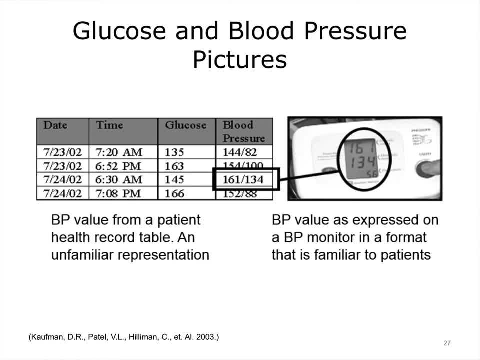 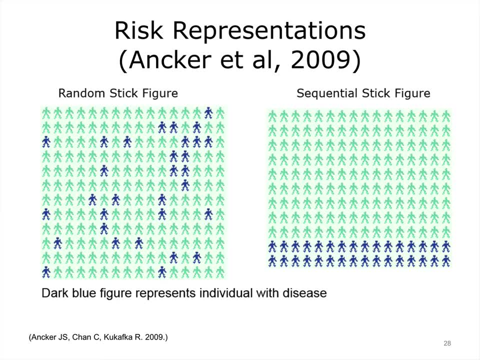 The representational effect has significant design implications. Jessica Anker has conducted research pertaining to communicating risks to patients. For example, if you're 50 years old and smoke, what is your risk of having a heart attack over the next 10 years? 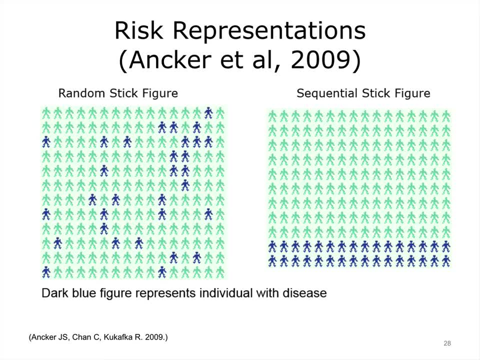 How does that differ from someone of the same age? Let's look at these two graphics. In the first one, dark blue stick figures who represent individuals with disease are randomly dispersed throughout a population. In the second graph, on the right, the dark blue stick figures are sequentially presented. 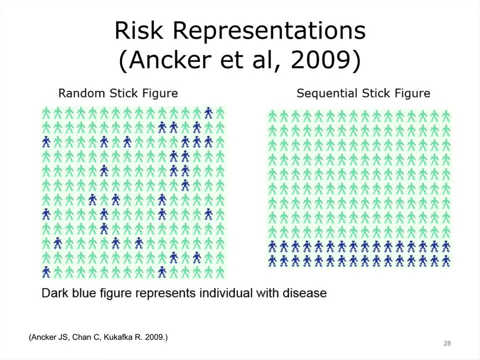 at the bottom of the screen. Although they represent the same probability, people are likely to interpret them differently. Dr Anker has experimented with different kinds of dynamic and static representations. In the second graph on the right, the dark blue stick figures are sequentially presented. 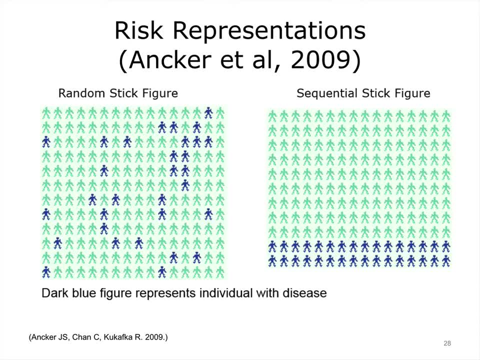 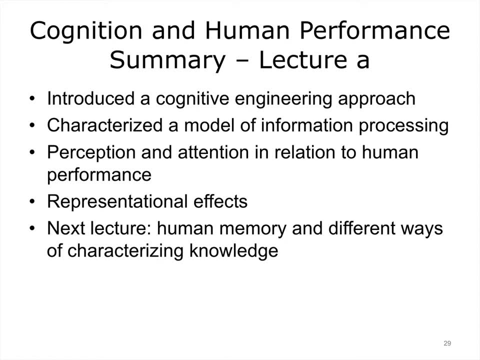 at the bottom of the screen. Although they represent the same probability, people are likely to interpret them differently. Dr Anker has experimented with different kinds of dynamic and static representations to determine which ones work best for different populations. This concludes Lecture A of Usability and Human Factors. Cognition and Human Performance. 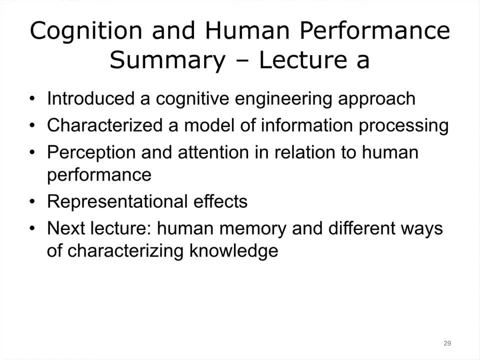 In this lecture, we explored different facets of human cognition in the context of a cognitive engineering approach. We introduced a basic model of human information processing and introduced issues pertaining to perception and attention. We also characterized how different kinds of representations can be used to determine.